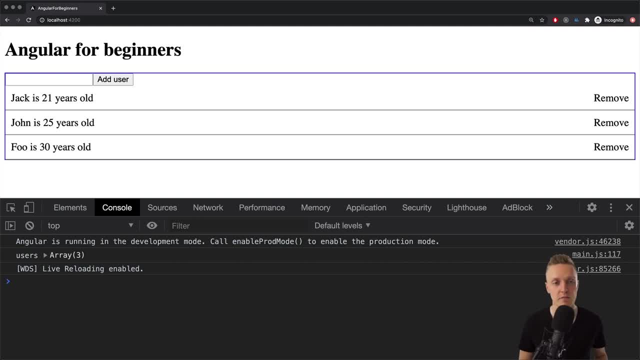 So what is routing in Angular and what is exactly frontend routing? So when we start building our web applications, normally we are building them with some backend server. So this backend server is running and we can access different pages inside different routes. For example, we have slash login. this is one page and it is rendered by backend. 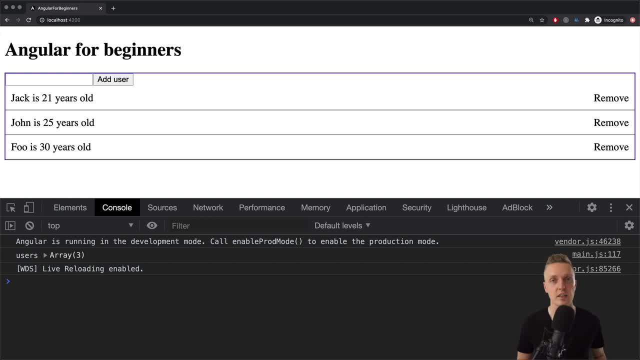 Then we have, for example, slash register. this is another page and backend is also rendering it. With frontend rendering and single page applications, it is working differently. So what is single page application? The idea is that backend server, instead of managing routing, simply always deliver for. 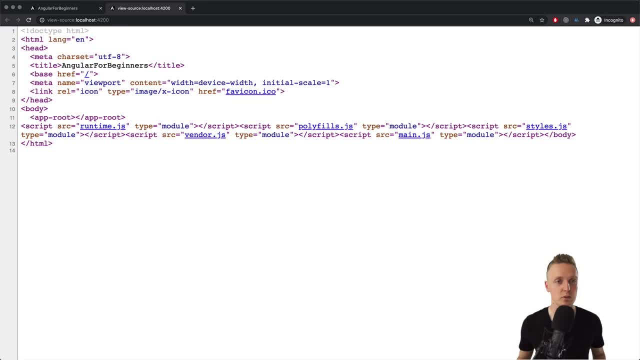 us indexhtml page And this is exactly what you can see here inside Angular. This is our HTML page and it is completely empty. The only thing that we have here is approot- this is where Angular is rendering- and scripts to call JavaScript. 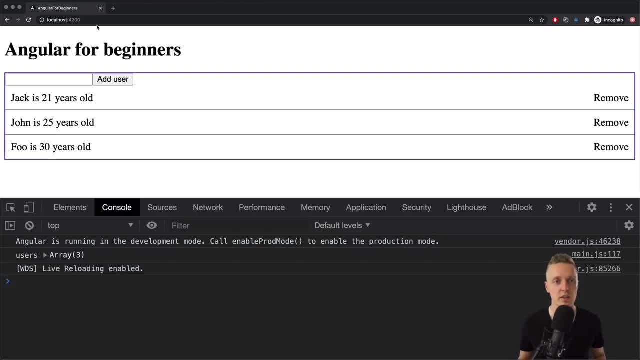 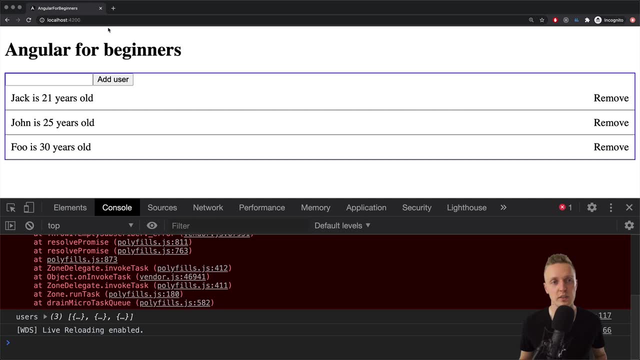 This is it, And the idea is, it doesn't matter in what round we're getting. like slash register, for example, backend doesn't do anything. Backend just simply renders this indexhtml page, But after this our JavaScript is being loaded and then JavaScript by itself thinks and renders. 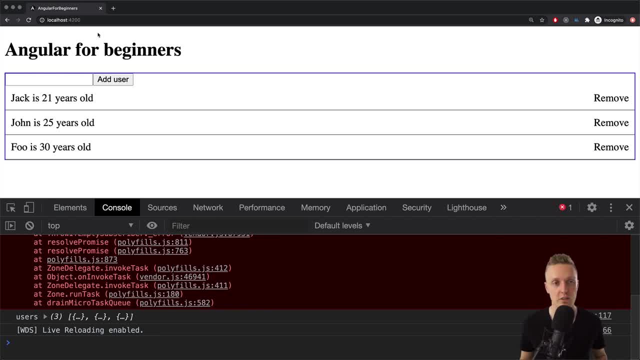 something which is related to this location, For example slash register, then our JavaScript will render for us the page which is related to register. Then we jump inside slash login and JavaScript is rendering for us login page. But the main difference is that this is happening without page reloading. 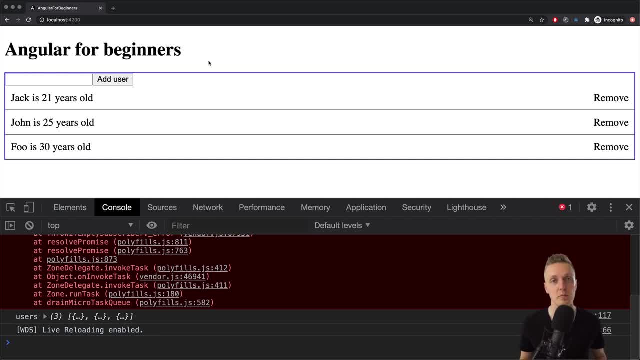 Because we don't have different pages. it's the same indexhtml page, but we just click on different URLs and we are getting different information. And Angular is working exactly in the same way with frontend rendering and we have everything out of the box. 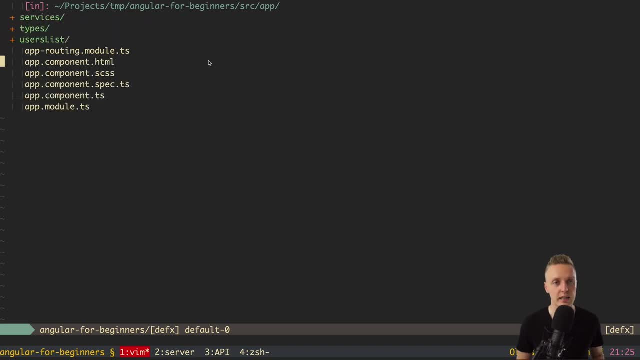 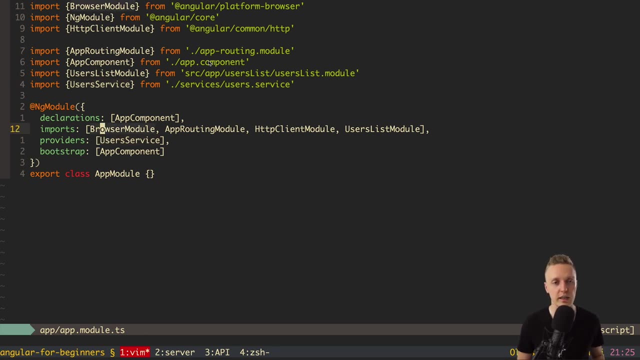 So let's check how Angular works, Angular is doing routing, and how we can use it. So let's jump in app module, because this is our first module and we need to have here our routing. And the interesting part here is this app routing module. 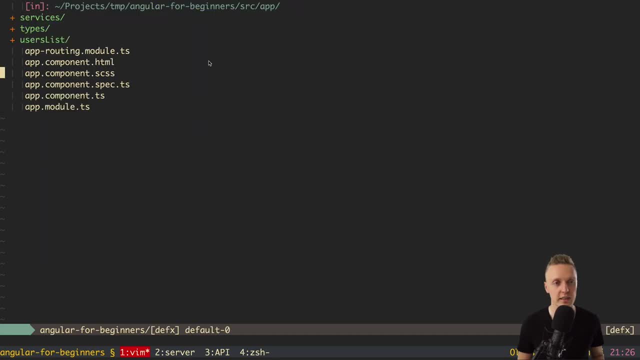 As you can see, this is just a module which is here nearby. So here is app routing module And it is like completely empty. we simply register here app routing module and we have here this impulse And this is like super important. 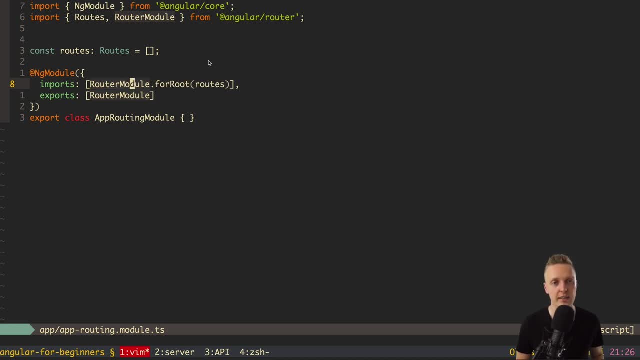 Because here we are registering our routes And here we are registering them with router module. This is the thing from Angular router. So this is the part of an Angular which is related to router And we are calling here dot for root and passing here array of routes. 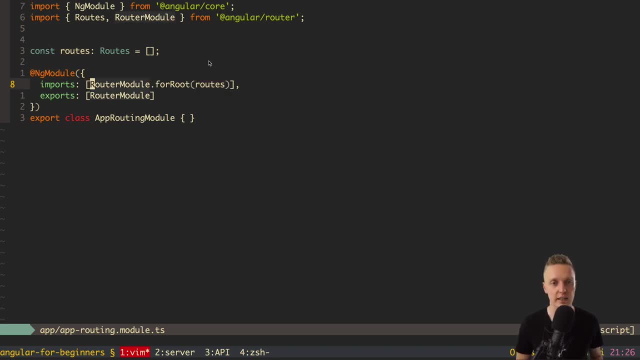 This is exactly how we are registering routes inside Angular And, as you can see, our routes array is completely empty. This means that we don't have any routes at all, But we can just create them and throw inside here. So let's check this now to know how it working. 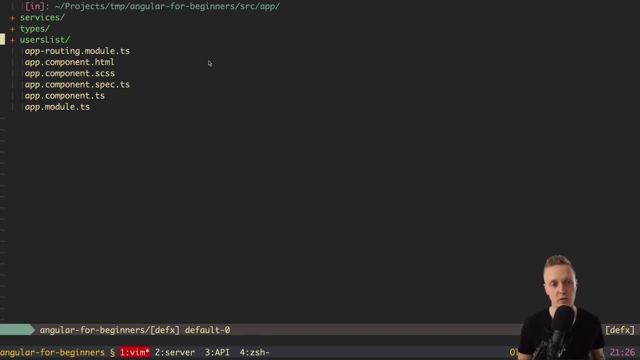 So the first thing that we need to do is create two different modules for two different pages, And let's make something useful in real applications. we have register page and login page, So let's add them right here. I will create new folder. 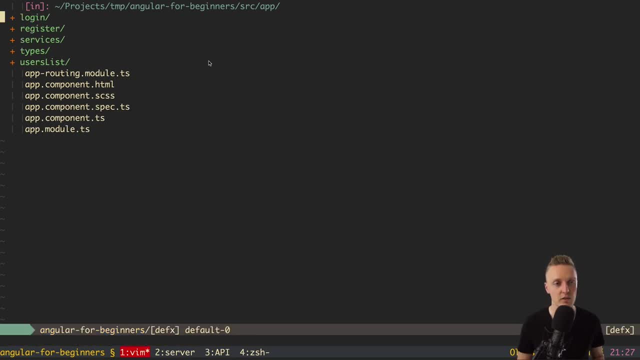 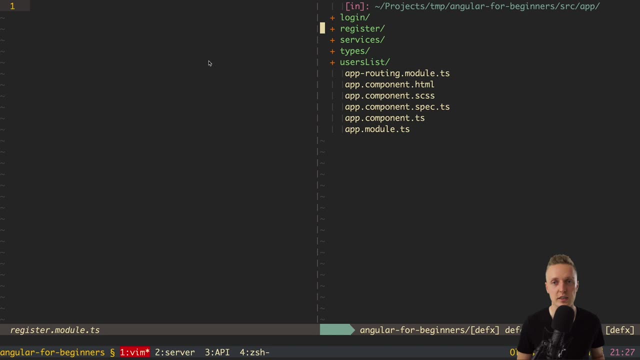 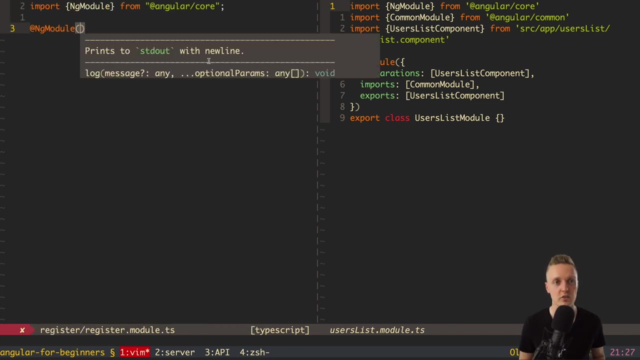 It will be register And I will create login folder. Let's first jump in register and create register module dot ts. And just to remind you, here we can check in users list, for example, how we need to declare a module. So first of all here we need ng module. 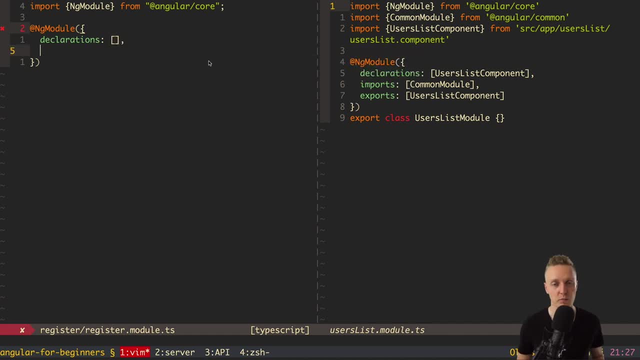 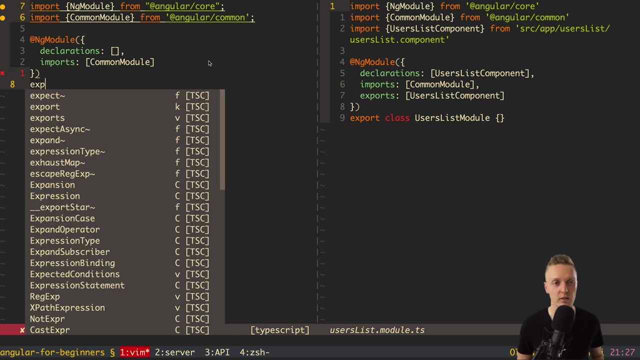 Inside we want declarations, And here will go our component when we will create it. We also need imports and it will be common module. With common module we are getting standard Angular stuff And inside exports we don't need anything because nothing will be exported outside. 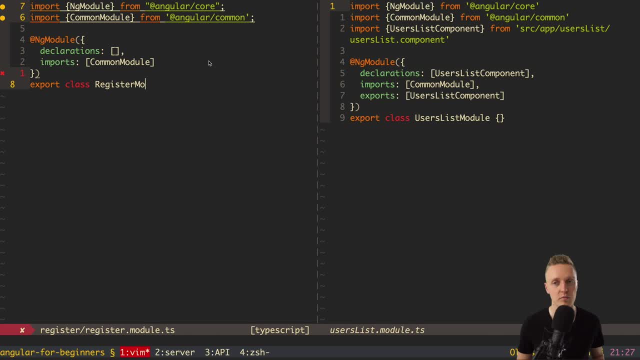 Now here we need to register our register module. This is it. So our module is ready. Now we need to create register component html and register component ts. Now let's jump first in html And right here, for example, simple div With content: register page. 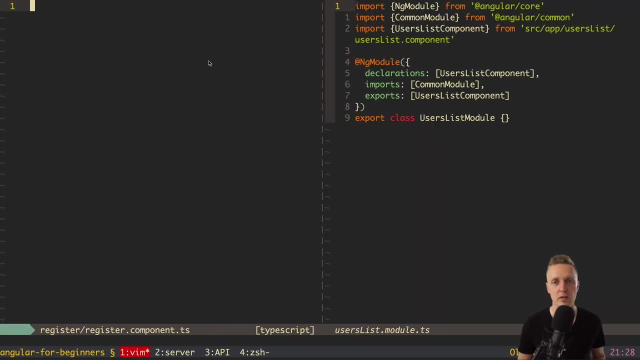 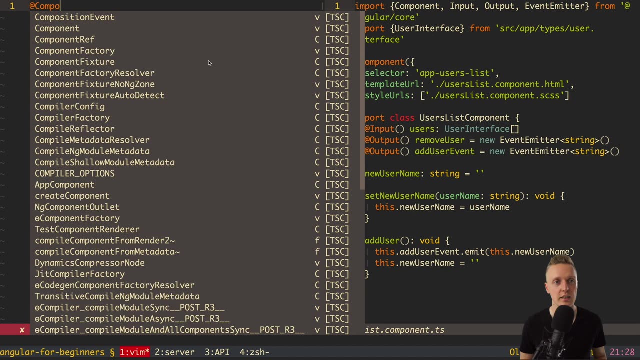 Now let's open our register, component ts, And I will open on the right, our users list component So we can check how we build it. So first of all, here is component and this is a decorator And we need to pass inside first selector. 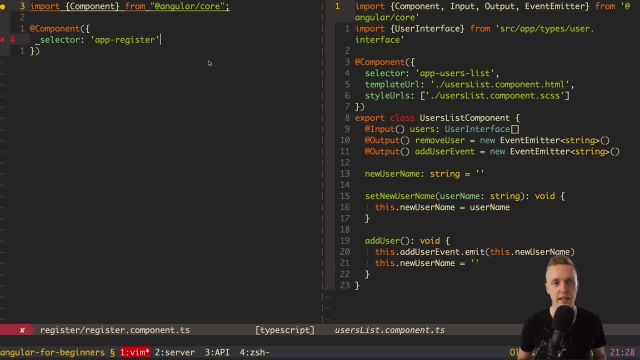 And inside here will be app, for example register, And just to remind you, we need app prefix To show that this selector is registered And it's not a library. Then we have here template url And in this case it will be register component html. 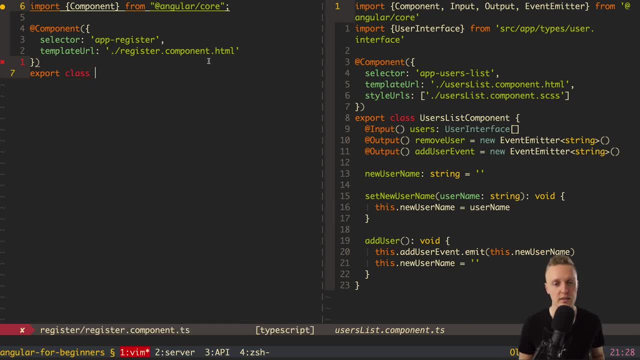 And here we simply want to register our class register component And we don't need to write any code inside our class. Now we simply need inside our register module to register in declarations: register component. So our component is there And our module is ready. 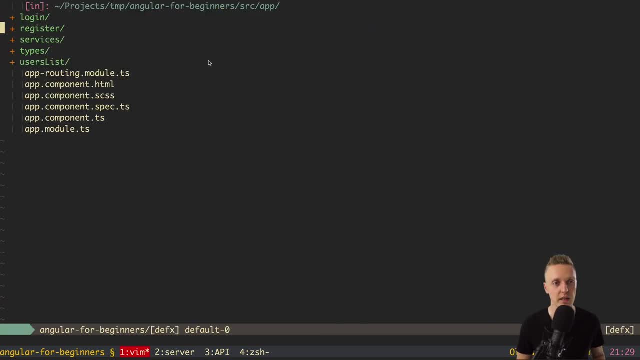 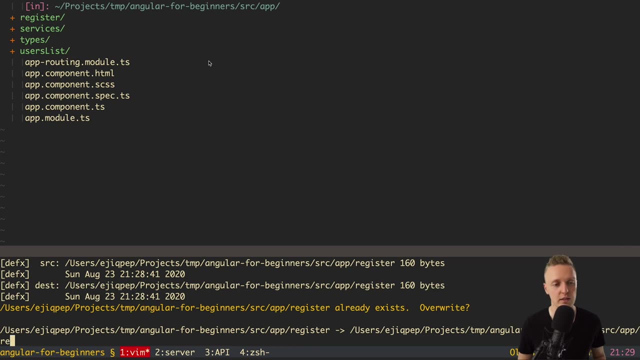 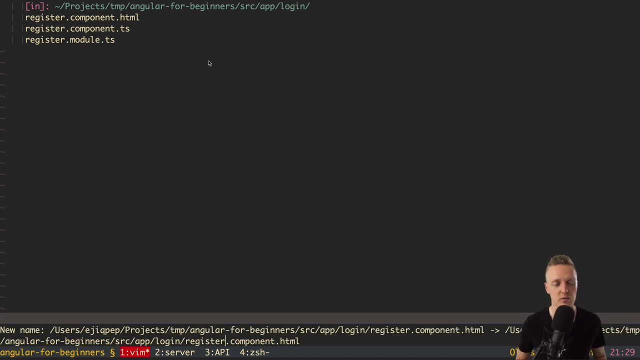 Now I want to do exactly the same with login page, So we can copy actually the whole register folder Just to avoid writing the same code, And we can rename it to login. Now we can change everything inside to login, So it will be login component ts. 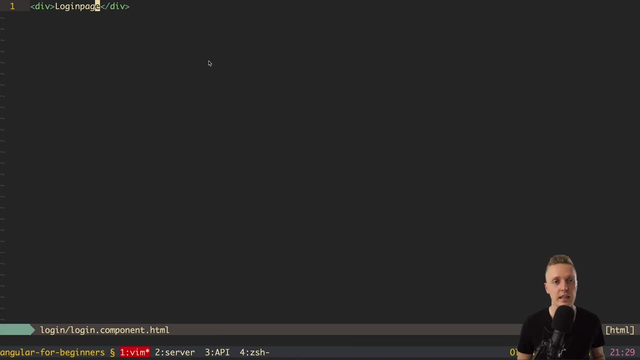 And here inside will be login page And here then we have our login component, component ts, And inside will be other selector. It will be app login And here will be login component html, And we need to rename our component to login component. 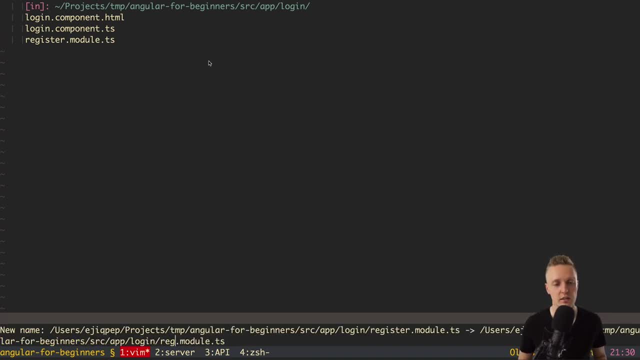 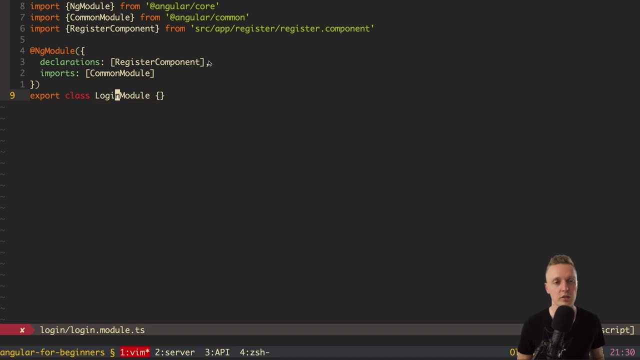 Now we need to change our register module inside login module And inside our module we want to change first the name- It will be login module And the declaration here will be login component, And then we can remove here register component. So we successfully created our login module and register module. 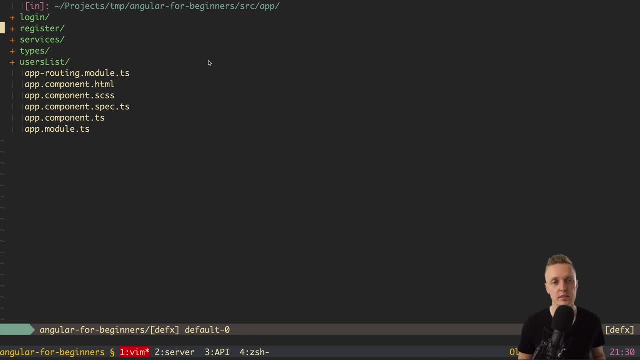 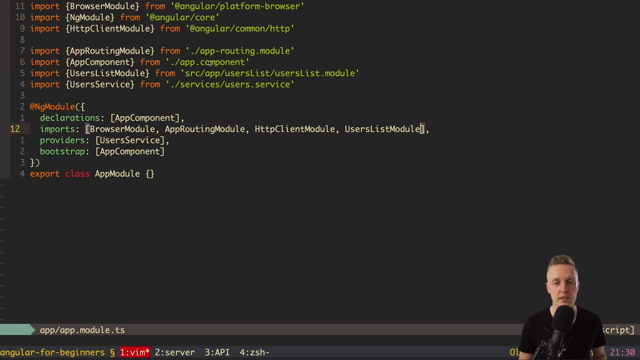 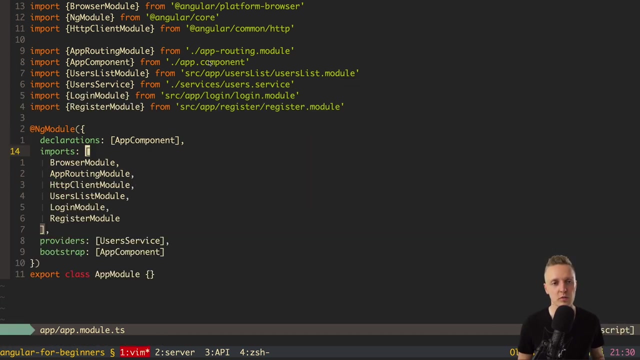 Now these two modules are created, but angular doesn't know anything about them, So we need to register them in app module, Because this is our main module. So here in imports we are writing login module and register module. So modules are registered, But if we open the browser, nothing is there, because these modules are not loaded in any. 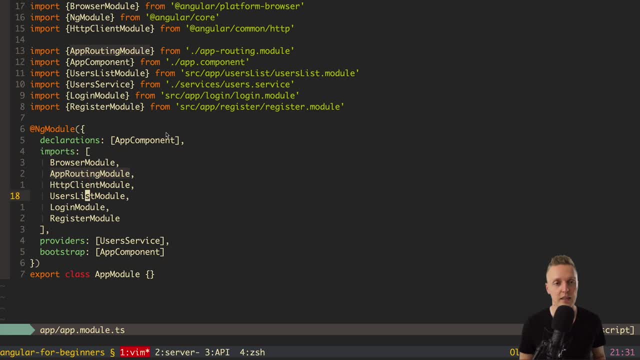 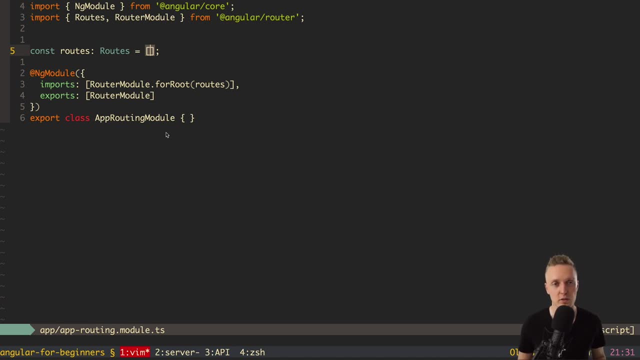 case, The question is how we can load them. So here we need to jump in app routing and define routes, Because we want to register one module with the route slash login and another with register. So here we need to add an object. And here we have two things. 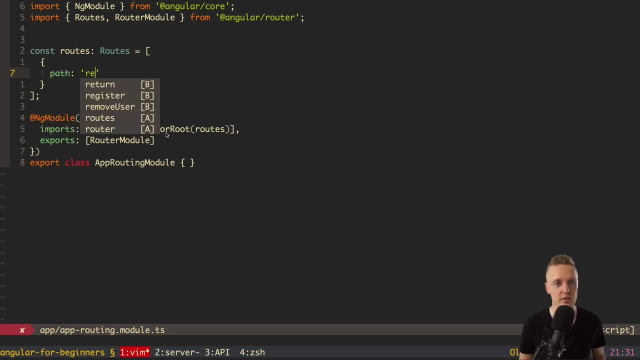 First of all it's path, And path is just a string, For example register, And just to remind you, we don't need slash here at the beginning. And now here is going component And in this case it will be register component And, as you can see, it is auto imported from our register folder. 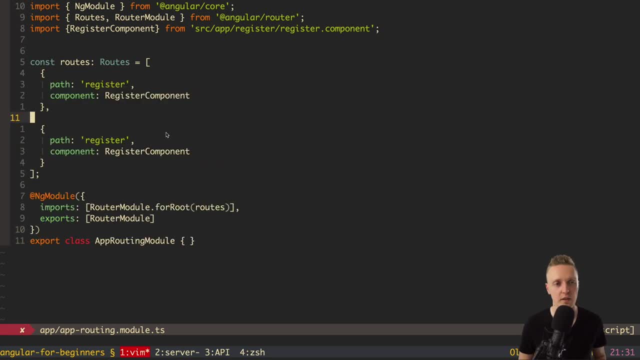 Now we need to do the same with our login. So here path slash, login, Actually without slash, And here we have login component. This is how you are registering inside our routes Components, What you want to render on this page. But what is really important is that it's not just enough to throw here inside components. 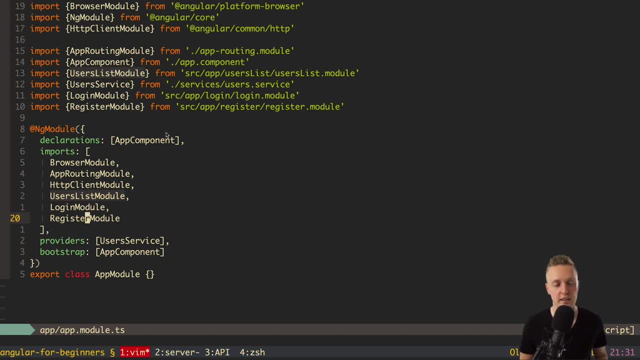 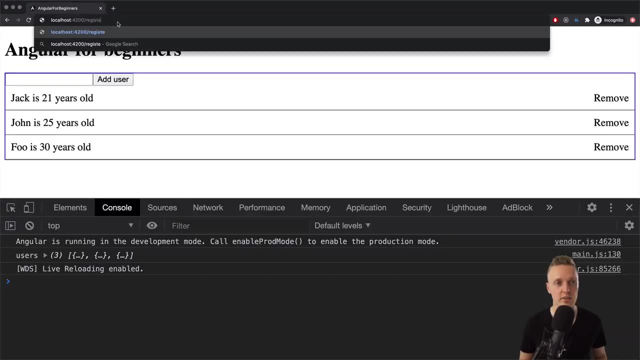 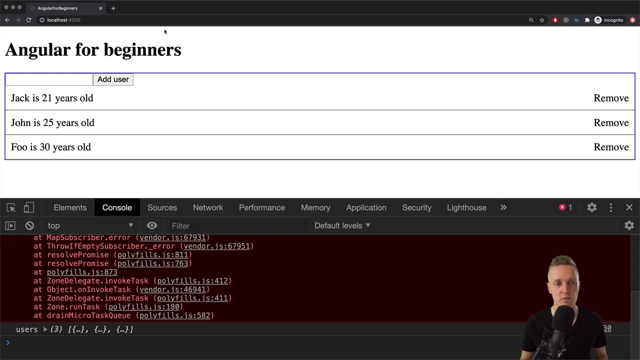 You really need to register your modules here inside imports list. Now let's check, we don't have any errors here And let's try to go to slash register page. As you can see, we don't get any errors from Angular, Because if we just write here, slash full. 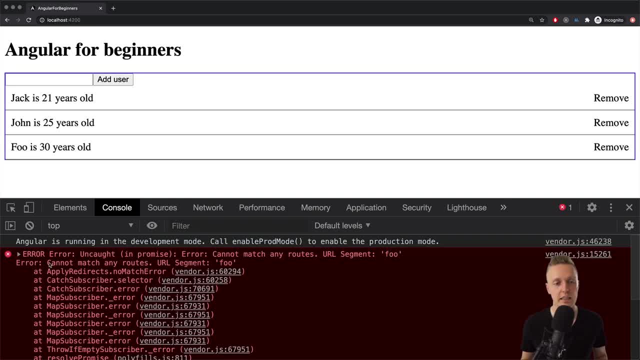 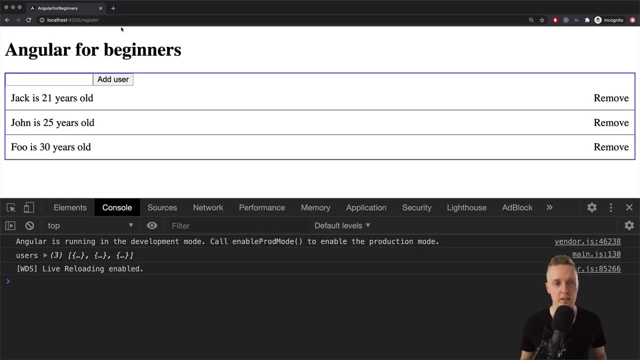 We are getting from Angular Angular. the error cannot match any routes And URL segment is full Because there is no registered routing for slash full. But when we jump in slash register First of all, we are not redirected back in home page And register is here inside path. 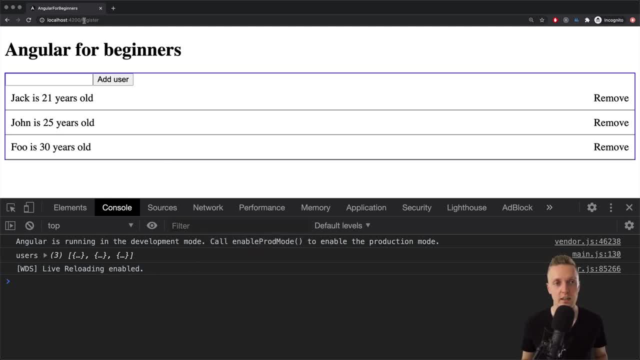 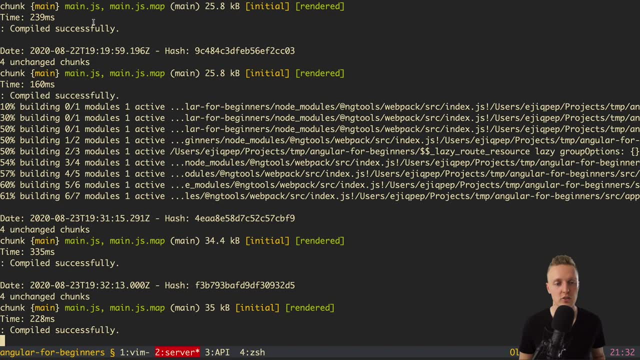 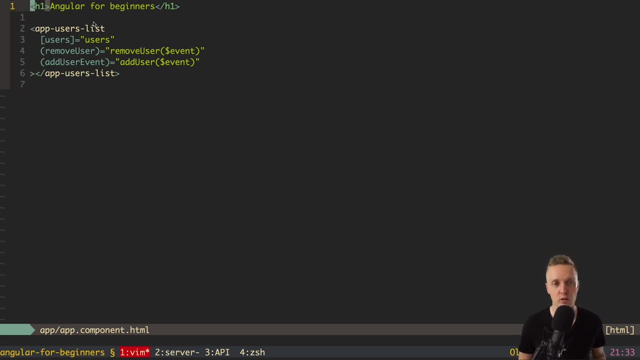 And we don't have any errors, Which means actually register module and register component are there, But we don't see any content. And the question is Why? Because if we look in app component HTML, There is nothing where register code and register component is rendered. 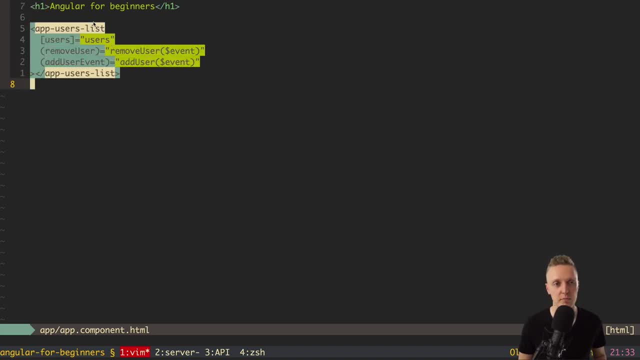 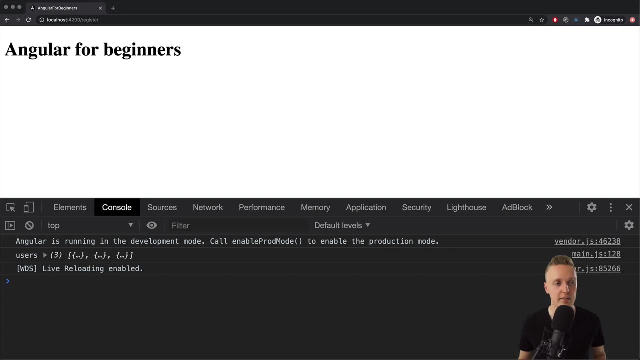 So we have here h1. And then we have here app users list. Let's comment it for now, Because just we want to see our two pages And actually there is an important component that we need to render To see the content of register page. 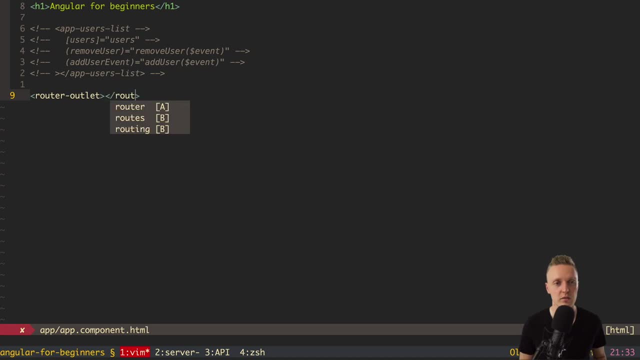 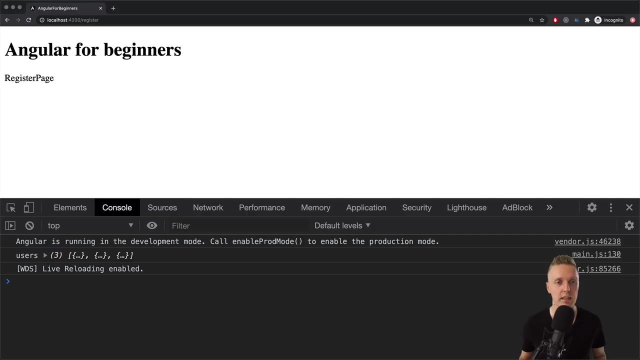 And it is called router outlet, So we need To open it and to close it here. So here is router outlet And this is exactly additional component from router module by itself To render the content of page inside the route. So when we look now inside our page, 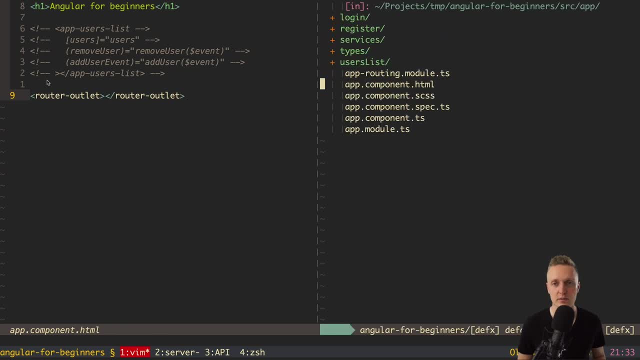 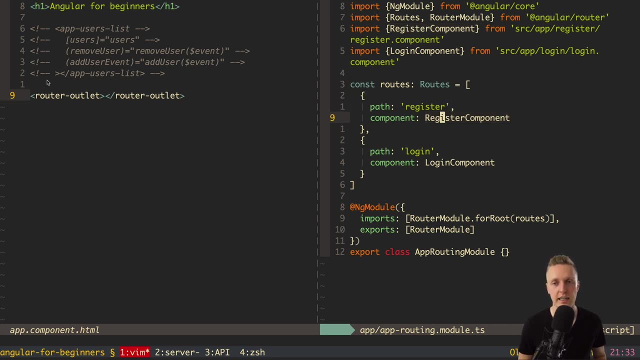 We see this register page component. So this is exactly what we had here inside app routing. So here inside route We have this path register And here is register component. And when we have here this component, Then angular understands: Okay, the path is slash register. 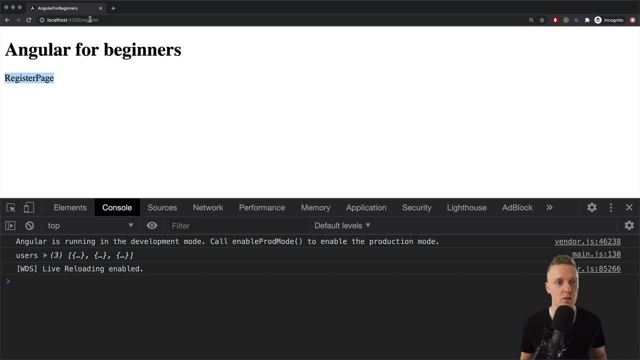 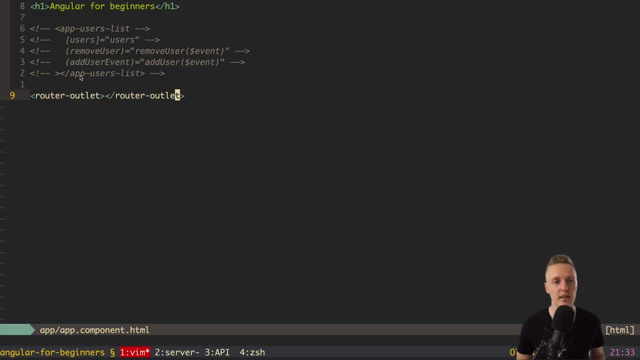 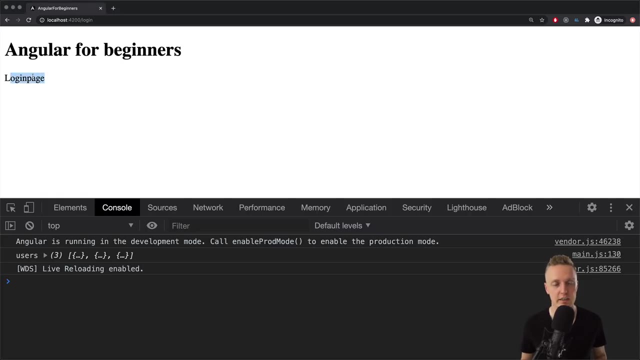 So it will render this register component. And now, when we go to slash login, Then, as you can see, it is login page And this is exactly how we are implementing routing inside angular, So we don't have actually page reload And everything is rendered here with javascript and not with backend. 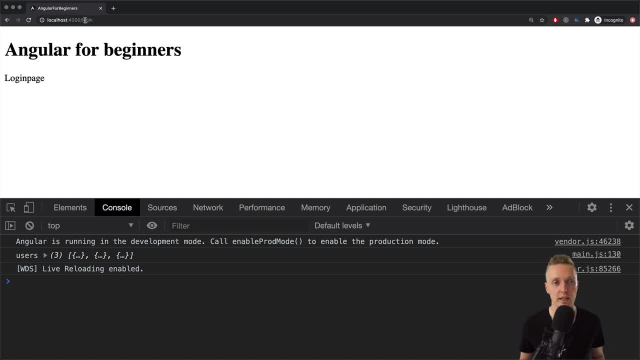 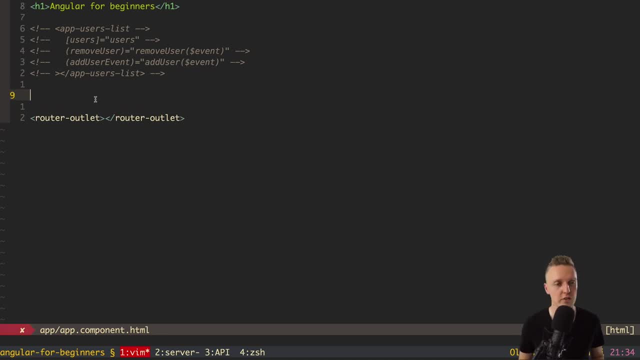 But of course We want that nice and clear, because we are simply typing in our url. Would be nice to have two links here on the top, for example, to switch between two pages, And for this there is a special component in angular which is called router link. 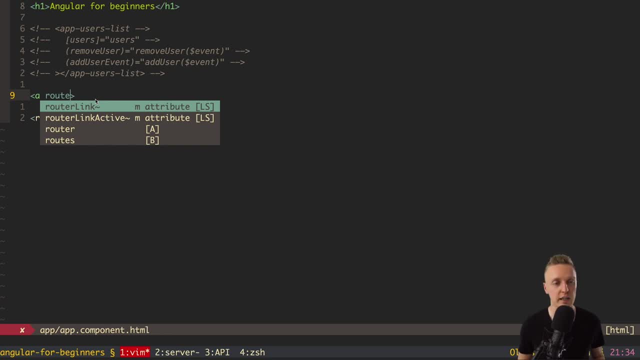 So we can say a like, always a href where we have in html, But here we have a router link and then slash login, for example, And here we want to close our a And here will be text of our url. Now here will be router link, slash register. 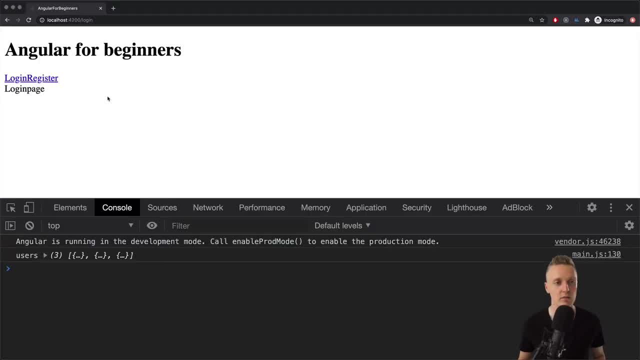 And here will be text register. Now let's look in browser. As you can see, we don't have any errors And here we have two links- Slash login and slash register- And if we will inspect them, They are looking exactly as normal links. 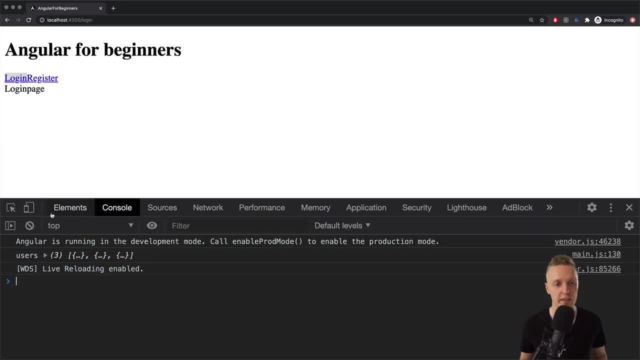 So here we have href, And this href was generated by angular. But what is important, When we click between these two links, We are getting different content on the bottom Because, basically, the url is changed. You can see it in a path here: 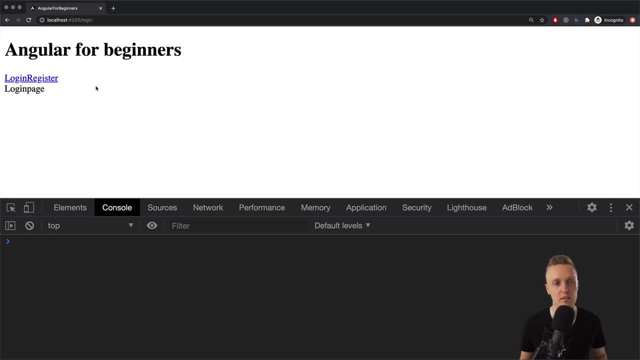 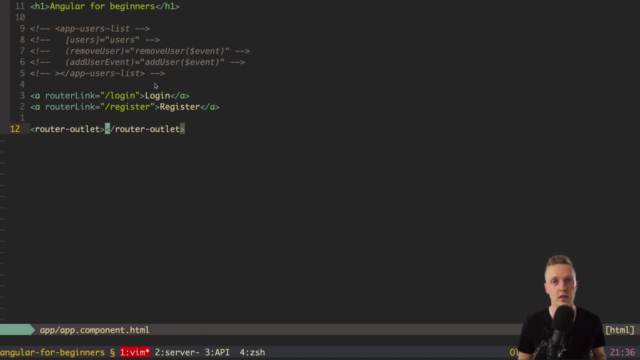 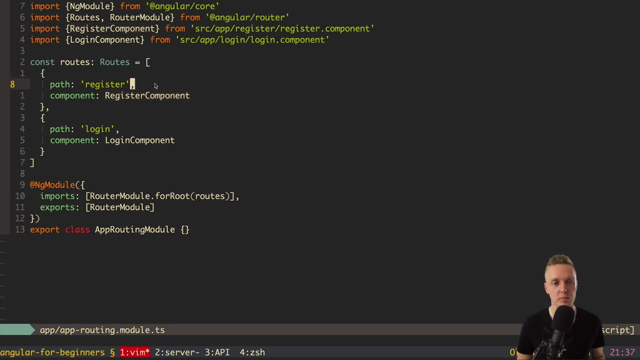 But the page is not reloaded, And this is exactly how single page applications are working. So, as you can see, angular managed everything on its own, So we don't need to do a lot of stuff. We simply need to register inside app routing our components and path. 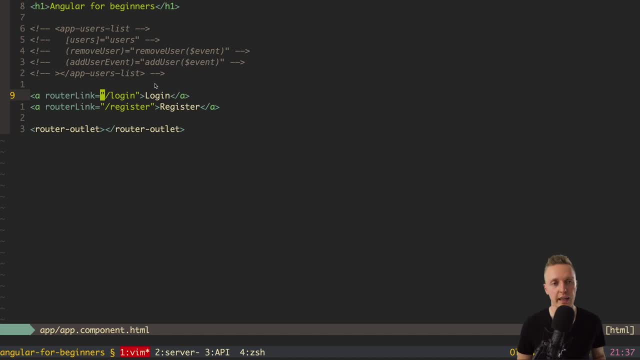 And then to use inside any place where we want A router link to create links to these pages. And what is important here? You might ask: what is router link and how does it work like this? And actually this is binding of properties, like we did previously. 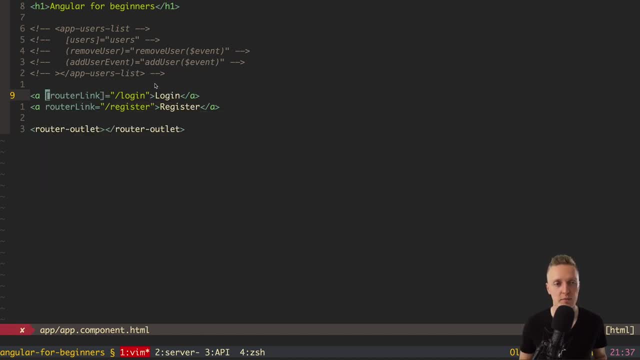 So you can remember that here we wrote something like this With square brackets, And you might ask why we don't use square brackets here. Actually, because we can omit square brackets if we want to pass a string. As you can see, Here we are getting the error now. 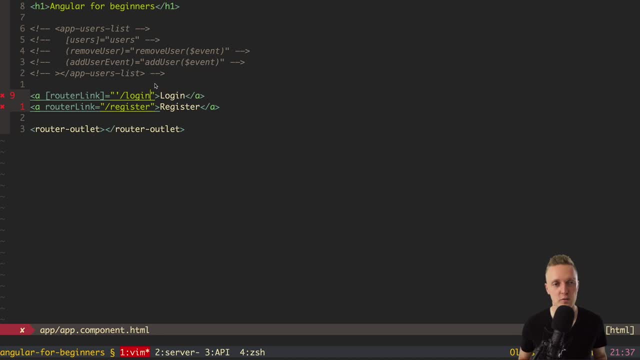 Because here we have square brackets And this means that here should be something to evaluate, And in this case it will be correct, Because now we want a variable here And here is the string, So you need additional quotes here. Of course, it looks uglier. 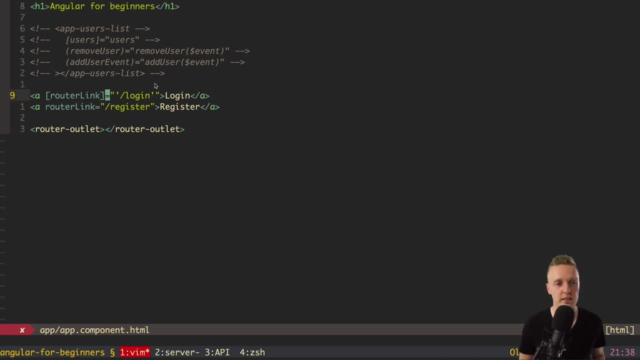 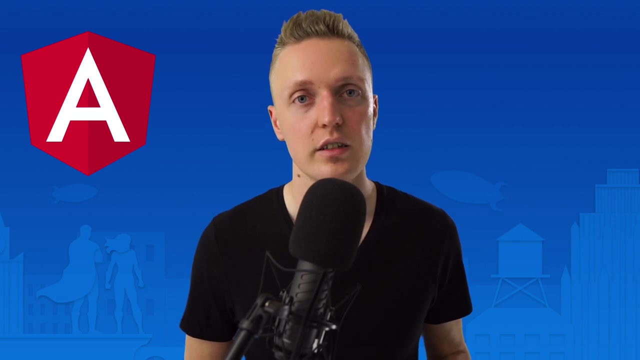 And it's more difficult to read. This is why we can omit this And just avoid square brackets if we want, here on the right, to have just string And not some variable or number or whatever property we want to pass. In this video you learned on the real example how Angular is working with routing. 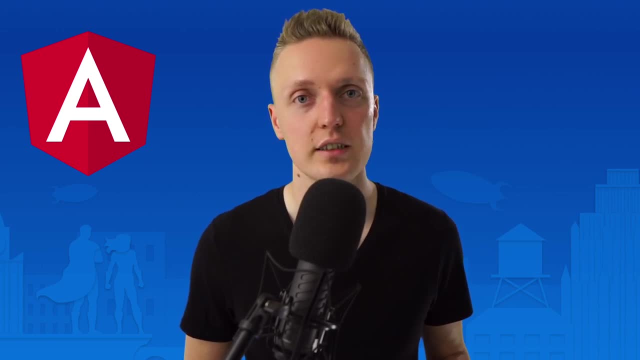 And as this is the last video in the series Angular for Beginners, I think now you should have enough knowledge to conquer my advanced Angular course, which is going 14 hours, where we are building real application from start to the end, Because videos with specific Angular features are not enough. 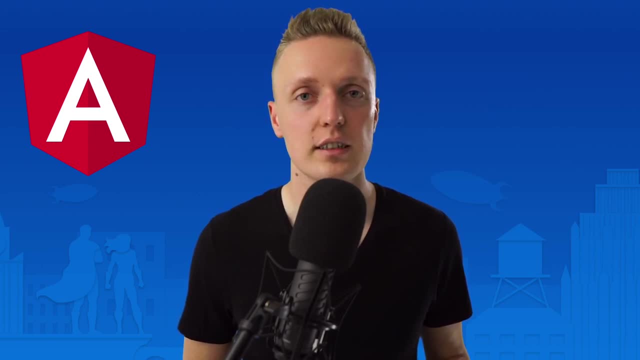 So I will show you how to do it, But you need to understand how to build the real application from scratch And I will link the link in the description below to this Angular course and to my other courses. And if you like this video and you want more content like this, don't forget to put thumbs. 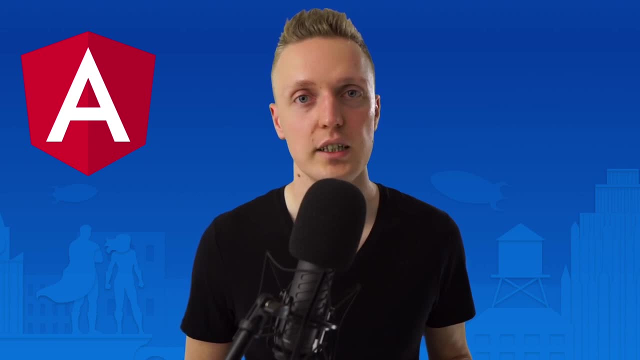 up and subscribe to the channel, And I will see you in my next video.